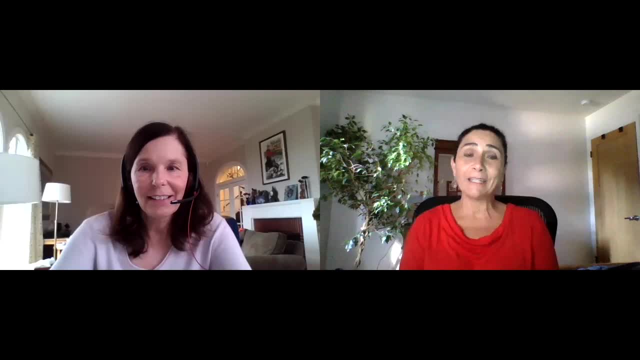 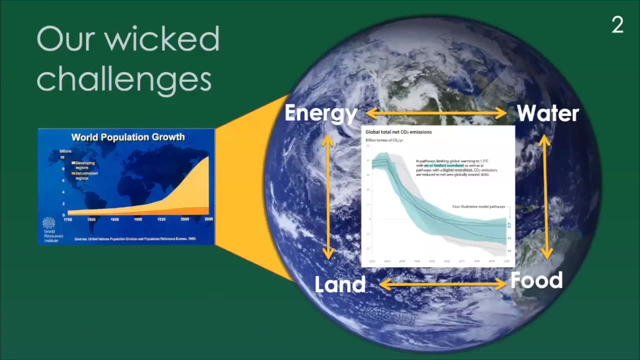 Thank you, Sarah and everybody, for being here today. As we heard yesterday, humanity is really facing a significant challenge with having to reduce carbon emissions from about the 40 gigatons per year we are having today to zero and also have a method to draw down CO2 emissions. 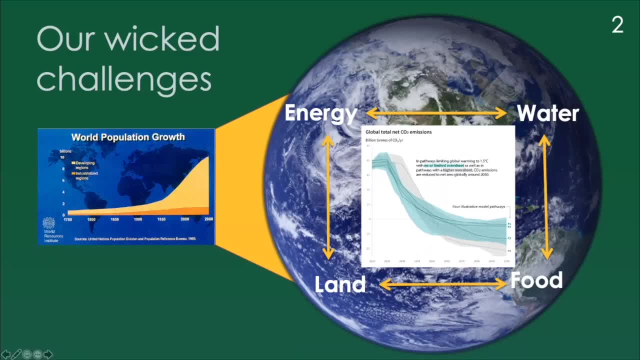 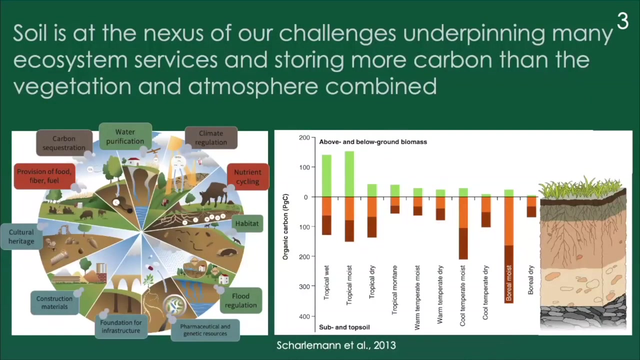 From the atmosphere actually to below zero in order to stabilize the climate, And we need to do that at a time when the global population is still rising and therefore their demand for energy, water, land and food is rising as well. We will hear today a lot of different solutions, and my goal is to drive you to one of the possible players in this fight against climate change. 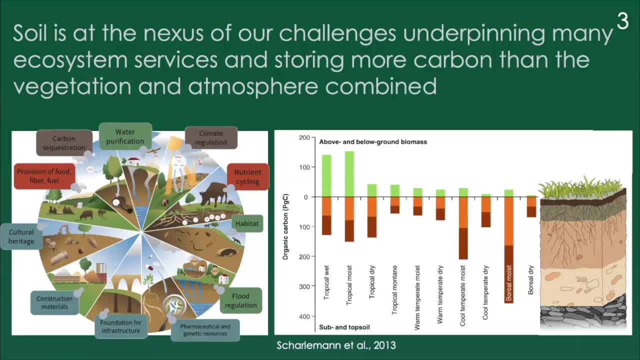 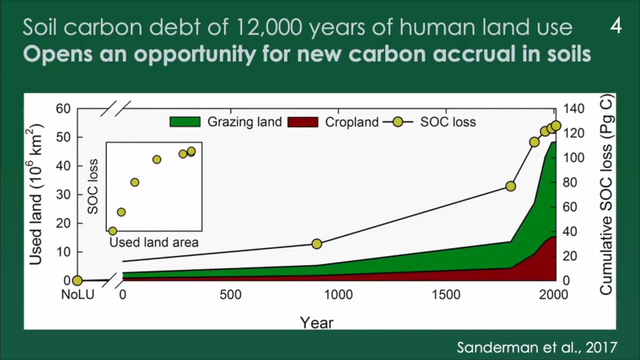 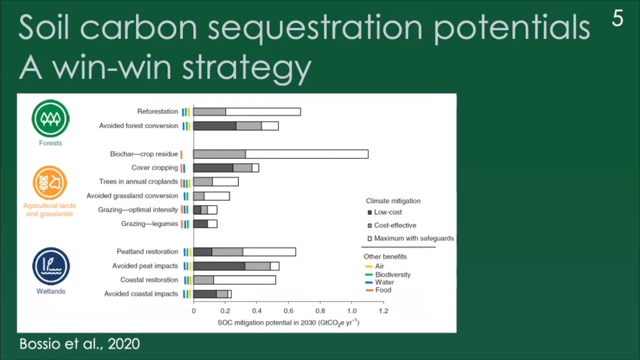 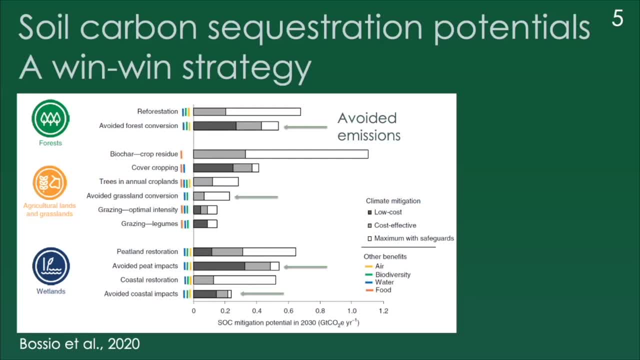 this is carbon that is currently in the soil. we just have to make sure that it doesn't go into the atmosphere. Those soil carbon sequestration strategies have several pros in particularly, most of them are relatively low cost. we know the technology that can be implemented with several benefit to hair, biodiversity, water, food has pointed in this. 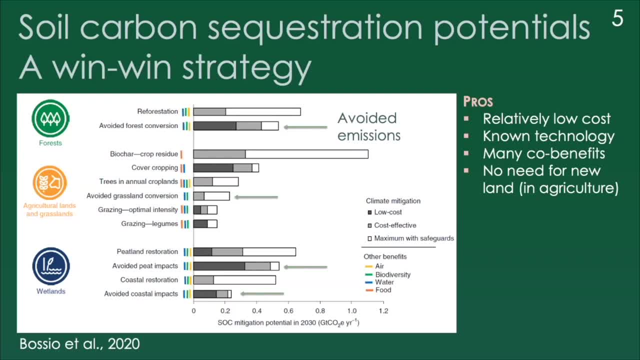 figure and also, at least for what they concern agricultural land, they don't really need more land, it's just a change of management in the land that is already under agriculture. There are some other questions, Several limits or cons or things that we need to. we need to be careful about when we look at 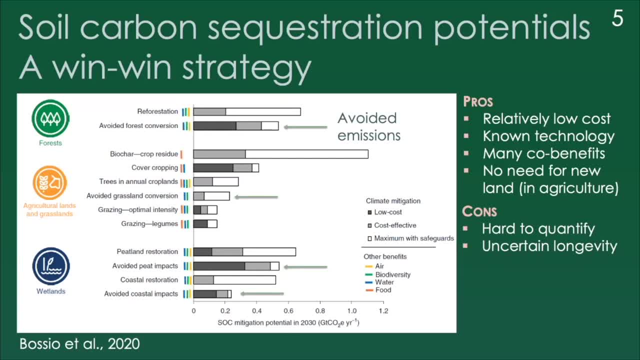 carbon sequestration, and those are in particularly the difficulties to quantify the amounts and the longevity. With those being the potential, there has been a lot of hype with doing it, but also a lot of criticism for whether those potential can actually be met and what I like to do with you. 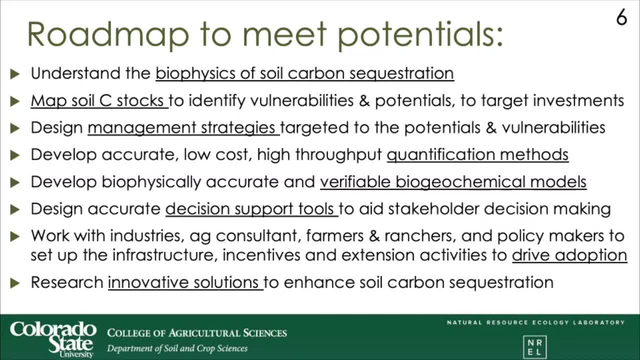 today is to ask you a question. I think the question is to go down what I think is a road map that can help us meet those potentials and that involved, first of all, starting from the science and the biophysical soil: carbon sequestration. use that understanding to have accurate maps or where carbon is in which pools are vulnerable. it. 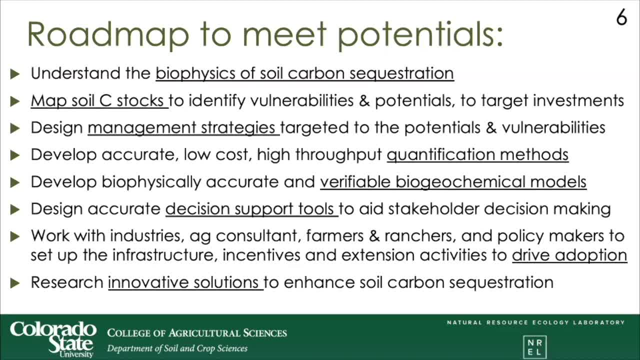 is so that we can target our investment and also design specific targeted management strategies for the different contexts. but also we need to develop accurate, low cost and high throughput quantification method and interface our our measurements with models that can use those measurements for actual verification and then include those models in decision support tools that stakeholders and 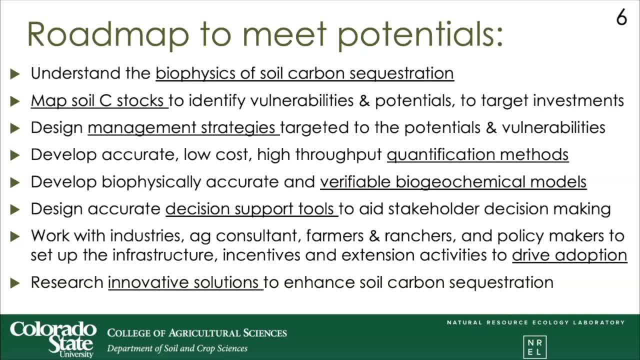 farmers and industries can use to make those decisions. And the most important point is that we need to work together and that's why I'm very excited to be talking to these audience today, because we do need to work with industry, our consultant, farmer and rancher policymakers. 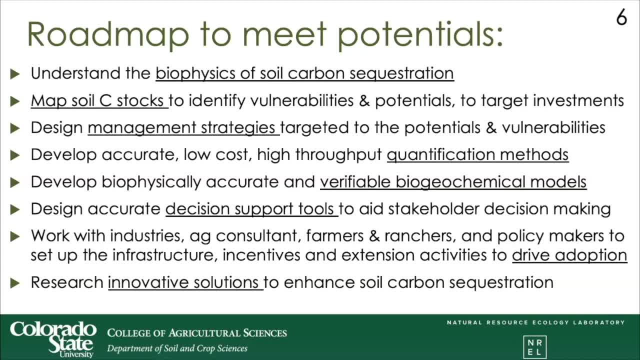 to get the infrastructure and incentive and and extension that can allow to scale up those processes. and finally, I also think that we need to keep do research to find more innovative solution. so this road map is also something. I also think that we need to do research to find more innovative solution. 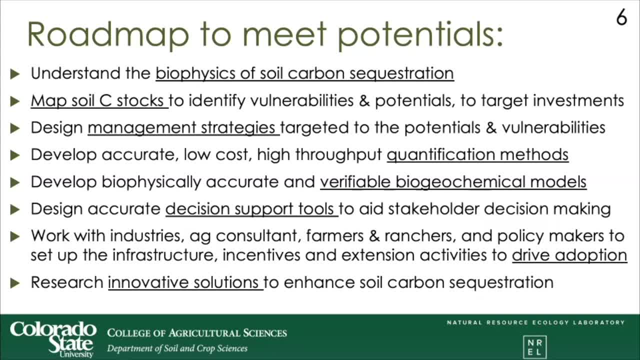 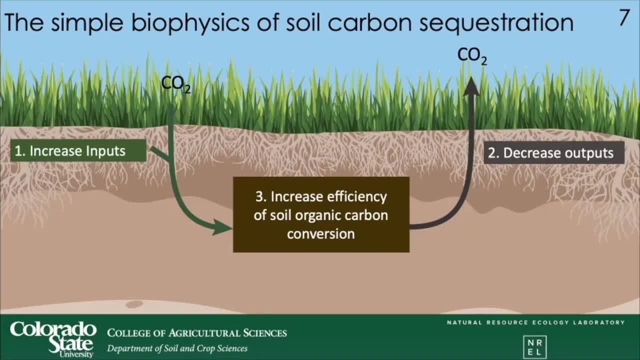 and results somewhat the outline of my talk. So let's start from the biophysics. The very simple biophysics is that if you want more carbon in soil, you have to increase inputs, you have to decrease outputs and possibly you can work with the efficiency. 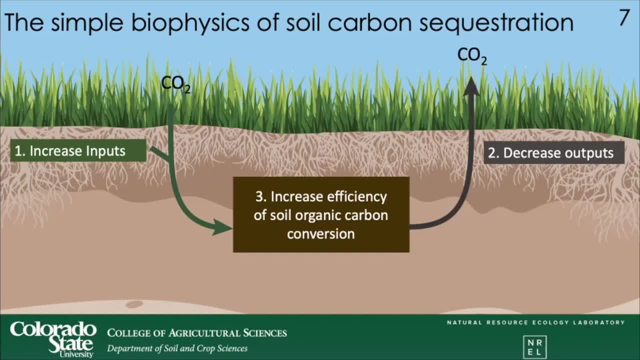 when which carbon is converted and increase that efficiency. We have a number of approaches that we can use to both increase inputs and decrease outputs, And some of them are very well known and can be implemented immediately. Other are more in the face of research. 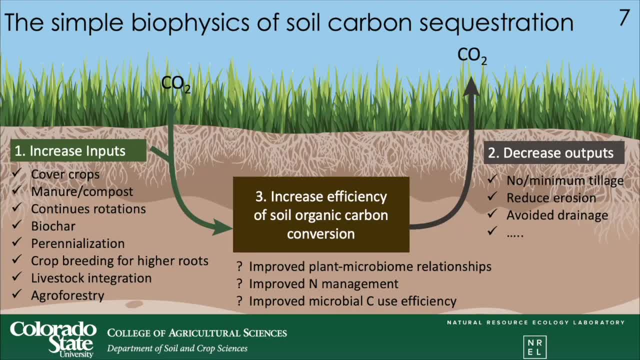 In particularly increasing efficiency is more in the face of research, but there is some very interesting work that show that we can do that by improving the relationship between plant and microbiome or also the nitrogen management. But what I want to do with you today 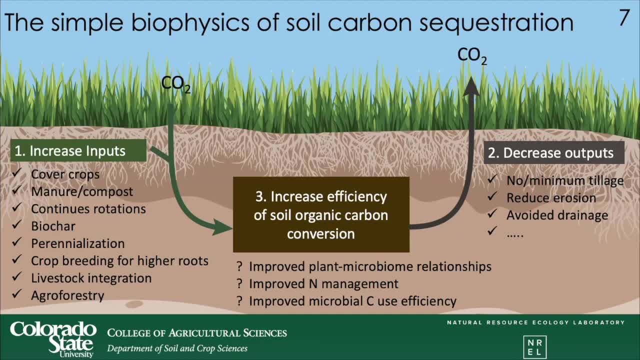 is actually stress the point that this biophysics is too simple. As a soil carbon scientist, I'm not gonna tell you about the complexity and all the difficulties of studying soils, but allow me to say that we do need to make one step forward. 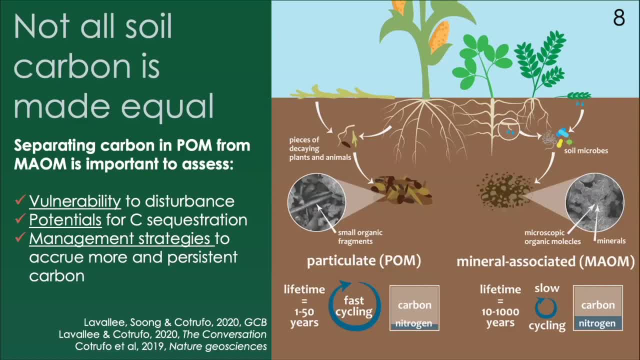 and acknowledge that not all soil carbon is equal, And the most important thing is to understand that the most simple approach that we can take and can bring to a way better stage, is to actually separate carbon, at the minimum in the two most distinct fraction, which are the particulate organic matter. 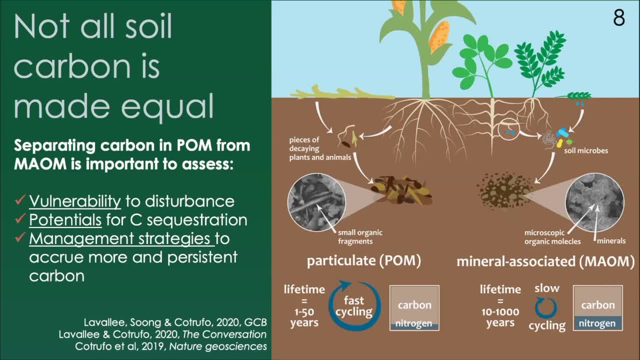 and the mineral associated organic matter. The reason why we need to do that is because those two fraction are created by different process And so different management respond and so different management respond. they will respond differently to management. They have a different permanence. 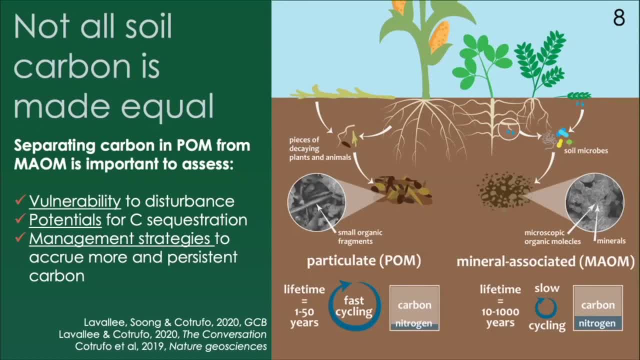 with the particulate being much having a much faster turnover, whether the mineral associated can actually stay in the soil for several, for several year. And the other difference is the different in nutrition. I don't in nutrients demand. I don't have the time to go into that today. 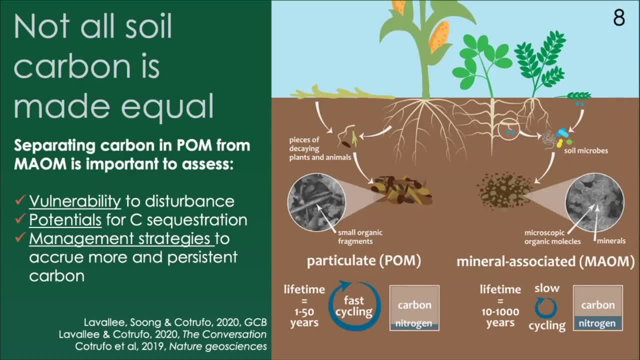 but for sure, the nitrogen demand of carbon sequestration is an important point and mineral associated require actually more nitrogen than the particulate gas, The particulate form mostly from plant debris and structural material, where the mineral associated this form from the soluble exudate through microbial transformation. 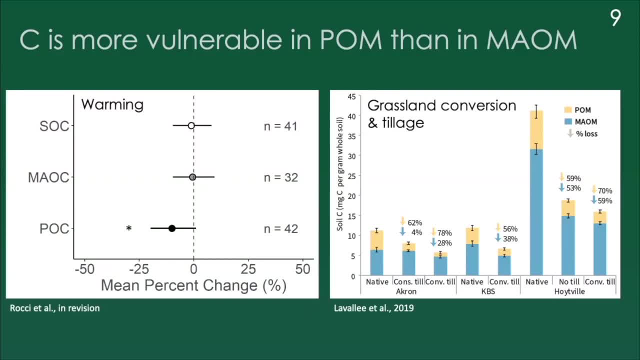 So why is it important to separate those two? First of all, palm is by far more vulnerable than now to decomposition, both to warming, And so when I was saying that we need to be to steward the existing carbon in soil, we mostly have to steward the palm carbon. 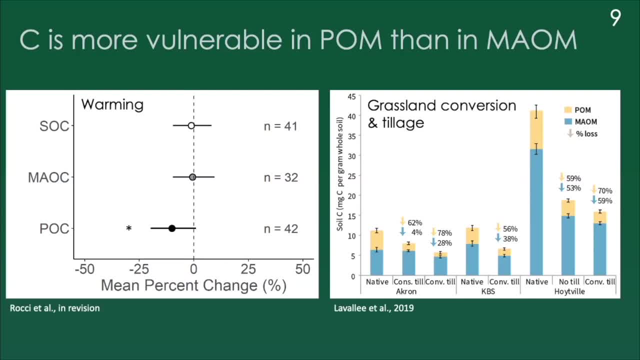 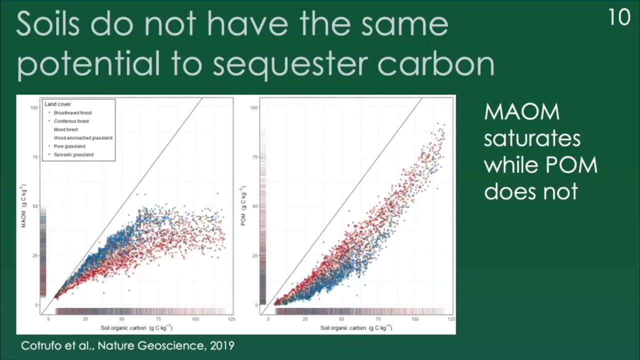 but also they have different vulnerability to management, with the, with actually the- the male being by far more stable and the palm being the the one that we lose, to the point that we have actually very little palm in agricultural soil, The other thing that is important. 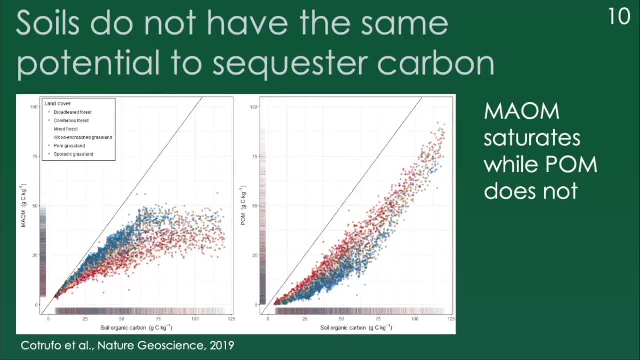 and we touched on it yesterday, is the concept of saturation, Since may require minerals to stabilize its saturate, and its saturation level depend on the amount and type of mineral in the soil, Whereas the palm on these other graph will not saturate, The good news here is that the majority of the soil 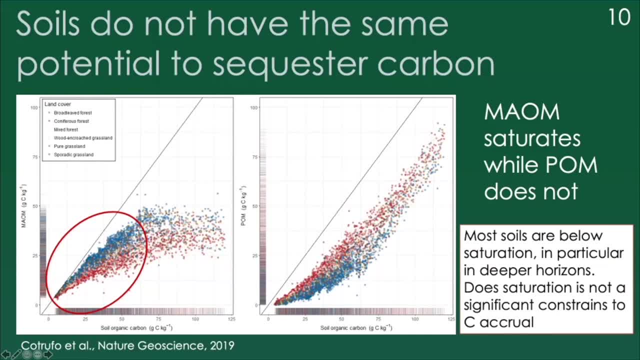 are far below the saturation level, And these are actually grassland and forest soils in Europe. The agricultural soils are typically down here, And so we do have a high potential for saturation, and right now we don't have to worry about saturation that much, in particularly if we focus on 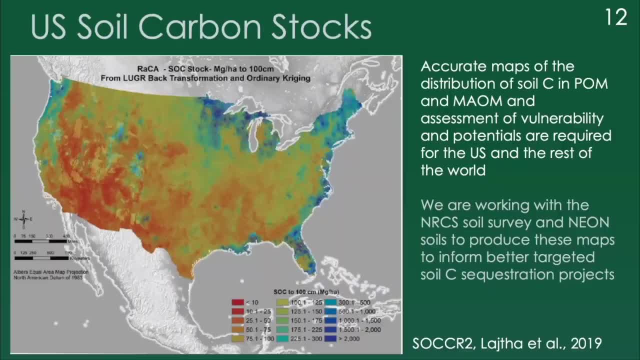 saturate on carbon sequestration in the deep soil, And the best map of carbon we have for the US is this: the. still, I like areas with high potential for carbon sequestration. I like areas where we really need to steward the land to. 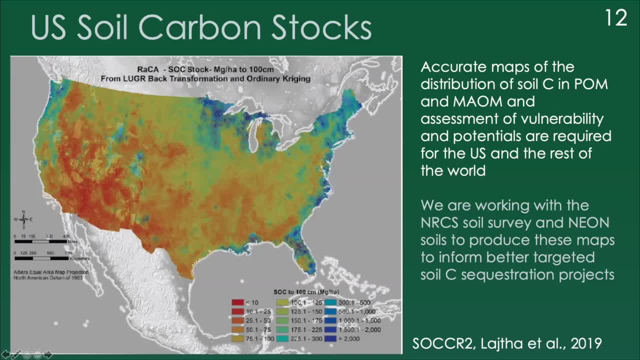 avoid carbon emissions, but we don't have an accurate distinction between those carbon forms that can further drive management, And that's something I'm trying to do in collaboration with the NHCS and me, and we are working on making a map of my own carbon. 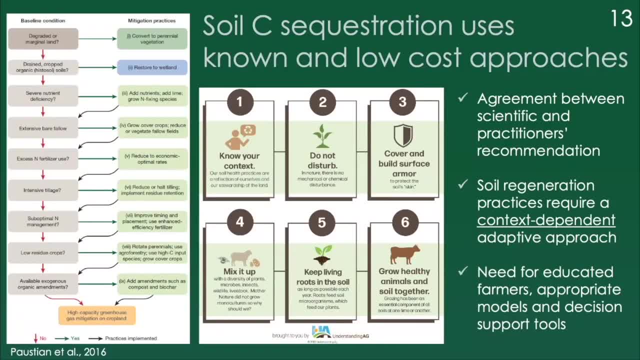 And with those understanding we can best drive management solution. Now, the silver line here that I'm very excited about is actually: we do know how to inform users about what they should do on land in order to increase carbon, And we know from 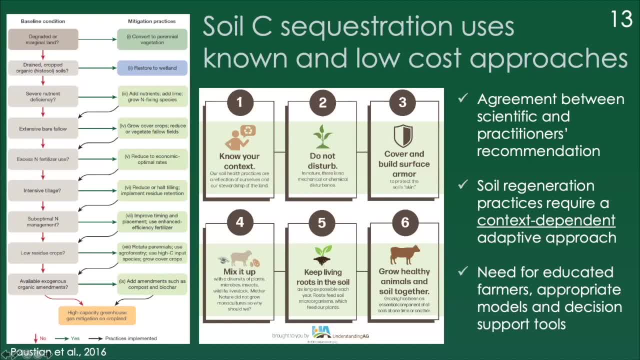 a scientific perspective, like this decision tree, that post and other published a few years back, and this is actually very similar to what the practitioner like understanding and people like Gabe Brown that has learned from his experience what it needs to do on his land to sequester carbon. 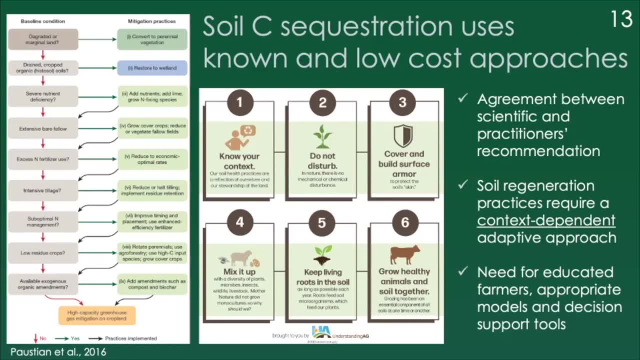 they are coming together and that, to me, is really highly motivating and exciting, And they both come to the point that carbon sequestration is, you know, something that has been shown is context-dependent, which means again that we need to have that background understanding. 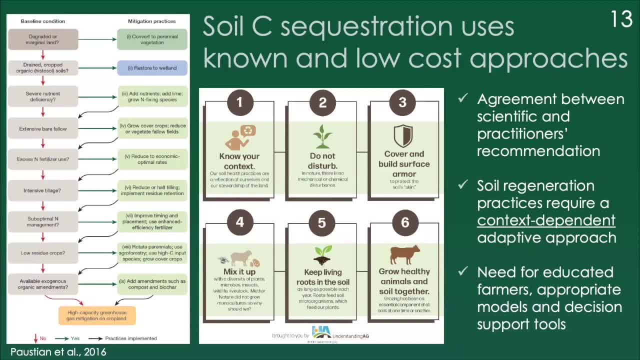 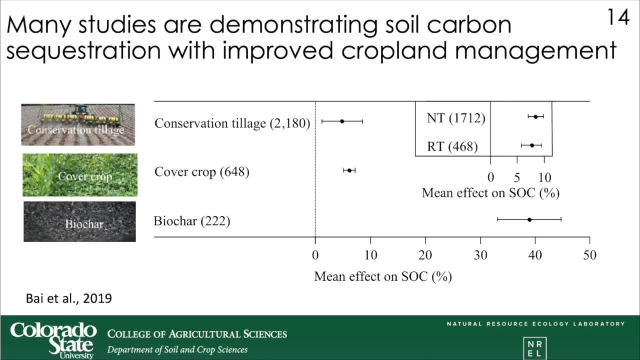 but we also need to work with farmers to educate them and give them the right decisions. So what are those practices that we can do? There has been a lot of work, a lot of meta-analysis. Maybe what rises to the top, says, in this meta-analysis, is the conservation tillage in 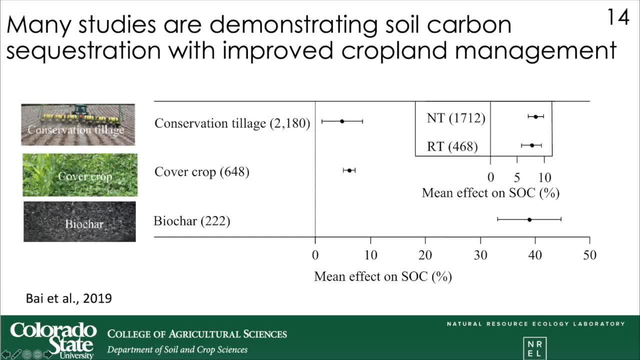 agricultural land has a solid benefit for carbon sequestration, particularly on the topsoil. Tillage doesn't increase carbon at that. Same goes for cover crop. Cover crop are really great at increasing carbon and improving its quality. mostly effective in the topsoil, Biochar comes. 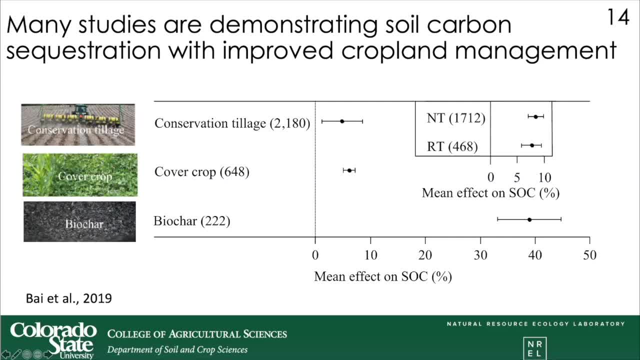 to a different scale because basically it's an addition of carbon-dense material in the soil that is recalcitrant and about 70% to 80% of what you put in is going to stay for centuries. But the problem with biochar is that we can't count from the moment we put it in. We need to 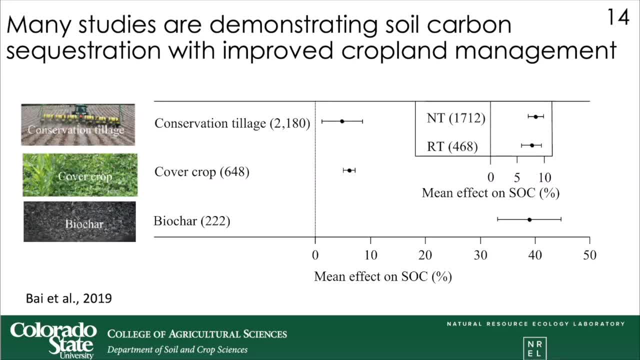 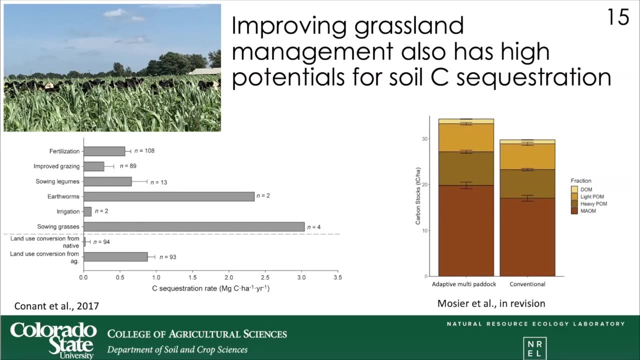 count the life cycle of biochar from the feedstock to the moment in which we put it on land, And so, depending on that, the carbon benefit can actually not be added. Also, grasslands can play an important role in carbon sequestration, So we need to be careful about that, And so we need to. 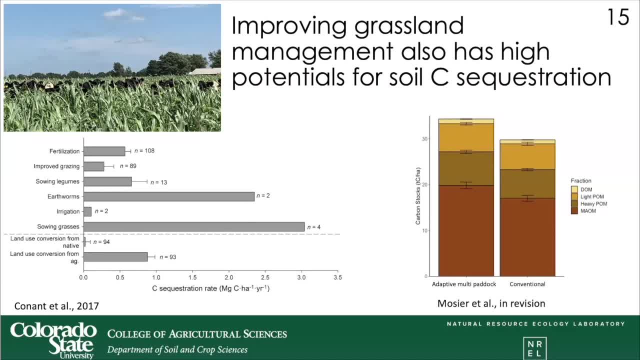 be careful about that, And so we need to be careful about that, And so we need to be careful about what we need to be careful about what we call carbon sequestration, And they also received a significant attention, and Rich Poon and others have done studies pointing to the potential. 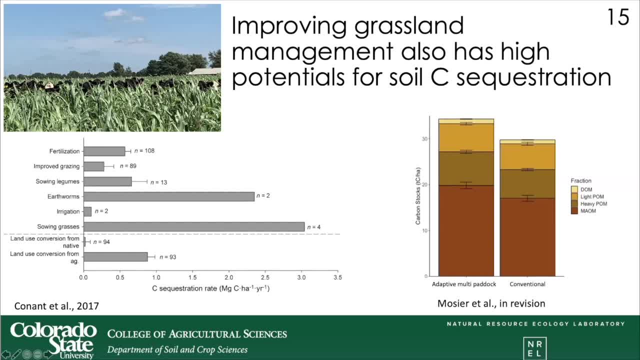 how different changes in management can increase carbon in grasslands. We just completed a study in grasslands in the south of the United States where we did the quantification but also the separation of maine and palm, And here I point out that by changing management to adapt, in multipandals For example, we could demonstrate 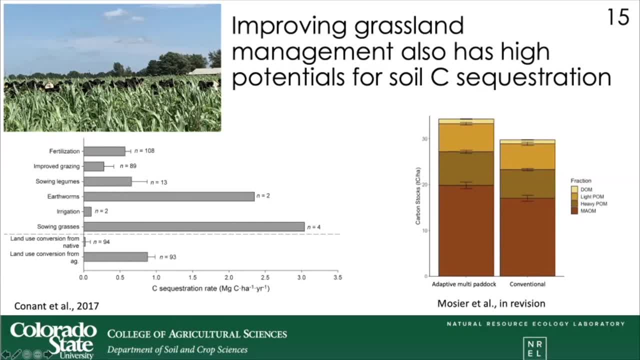 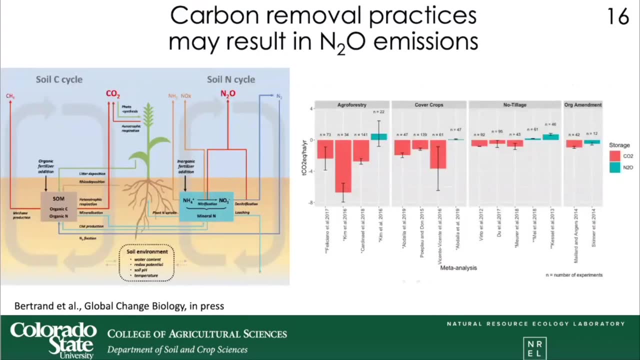 straight then. not only they increased about nine tons per per hectare over a period of about 10 years um, but also the majority of the carbon was was occurred in maryland, so it was mostly, but of course not everything is so easy and um carbon sequestration might lead to n2o emissions. 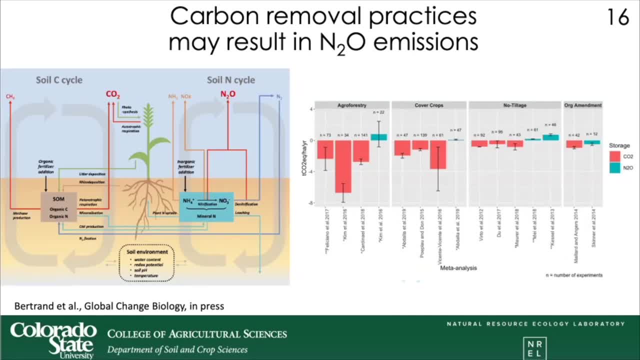 and i know that david will talk more about that later, but that's something that we need to be aware of, and this is actually a meta-analysis that hasn't come out yet in global change biology, oh, but it will soon, and and it shows that, for example, for some of the carbon sequestration- 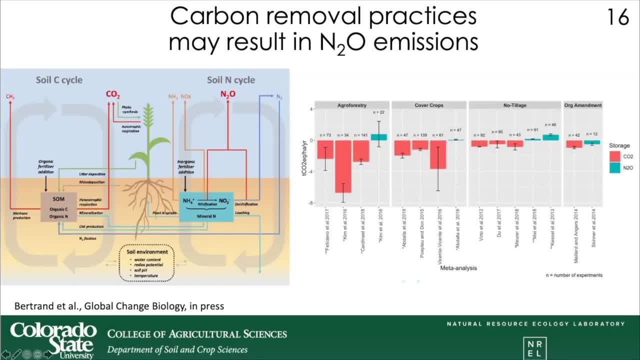 for the, the practice that accrue carbon. they might release um, n2o, and so that is something to watch out. all of these studies- or the majority of them, um- have been done mostly as independent studies on experimental stations and some on farm work, but what we really need to be effective is to move to a larger scale. 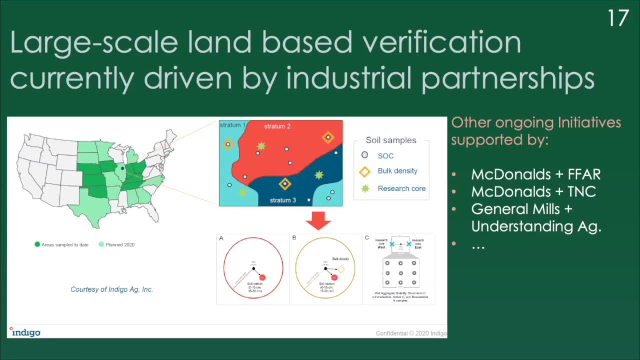 and i am very excited about the fact that industries are actually jumping into this and helping us to move to a different scale. um indigo is playing a big role in this work and they have launched an initiative for which they are monitoring carbon sequestration in a. 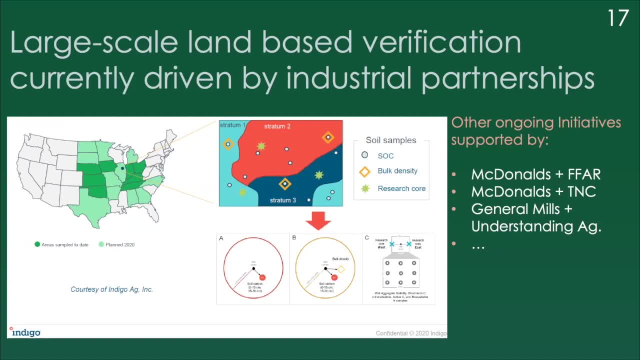 variety of farms and all across um, the, the mid us. but other similar initiatives are currently being done and supported by general meals, mcdonald's, um, tns, tnc and so forth. so that's really exciting. but the moment in which we change scale, it means that we need to start analyzing thousands of 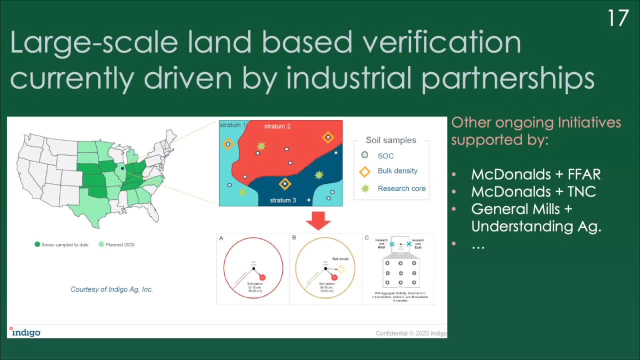 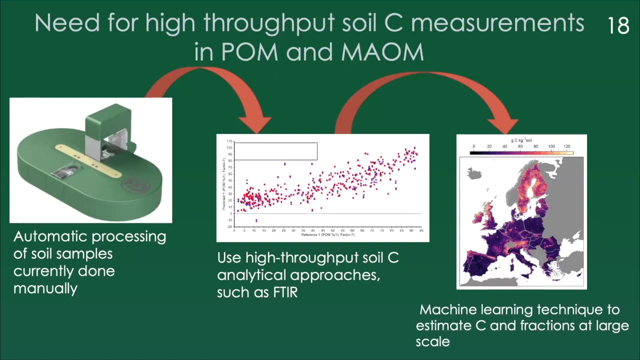 soils, and so you know that's i. i have a lab in which analyze soils, and the moment in which i'm telling you that you not only have to quantify carbon, but you have to quantify carbon in mailman home, i also understand the importance of uh, of providing um a solution for high throughput. 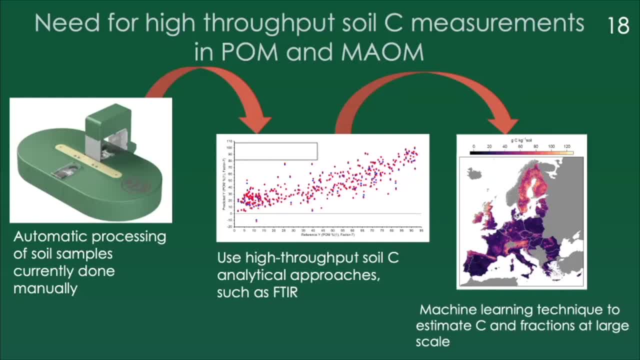 analysis, and that's something we are doing at csu, where we are working with engineers to design instruments that can automatize the, for example, the soil organic matter fractionation in my own farm, and couple those analysis with mid infrared spectroscopy and other methods that can um that they can analyze with a high 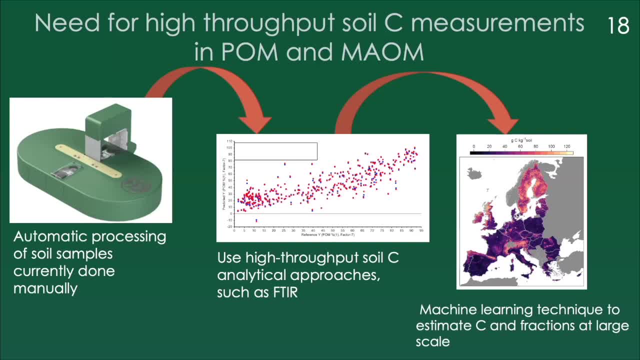 throughput and low cost, high number of soils. and then we need to work with the continental scale database and statistical approaches like machine learning to really get to those maps. so that's something that i'm very excited and we are working on in my lab. finally, these kind of models that need 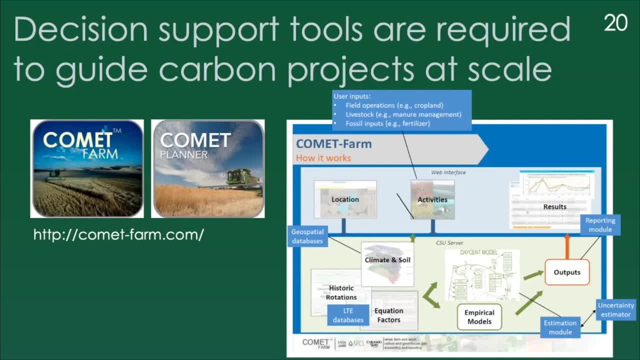 uh to really be used to process uh, the, the, the, the data and the, the, uh, the energy and the, uh, the, uh, the, the, the, the data and the, the uh, the, uh, the, the, the, the data of the of the energy, uh and of the safety, and the um data and the so much that's available and uh that can often can. 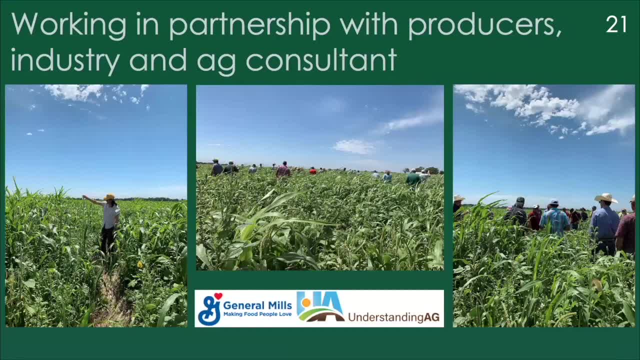 be used to, uh, to actually work with other forces in the field, so which have provided a much more important to have a pretty good interaction with other parts of the um. this the nature of our. I'm collaborating with General Mills on a project on grain farms in Kansas and we hope to expand it. 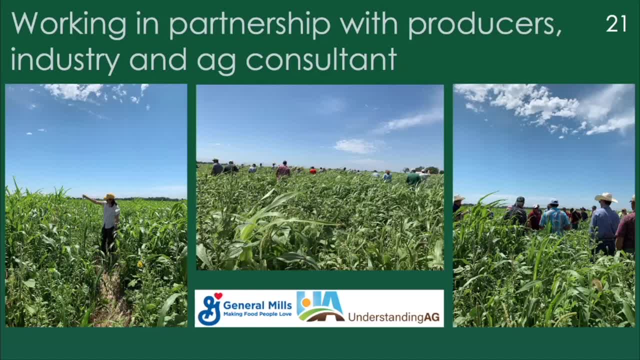 to Oklahoma and Nebraska And it was great to work alongside ag consultants and farmers to really see and demonstrate on the land those regenerative practices and how they can again be a win-win not just for the soil health and ecosystem health but really for the economics. 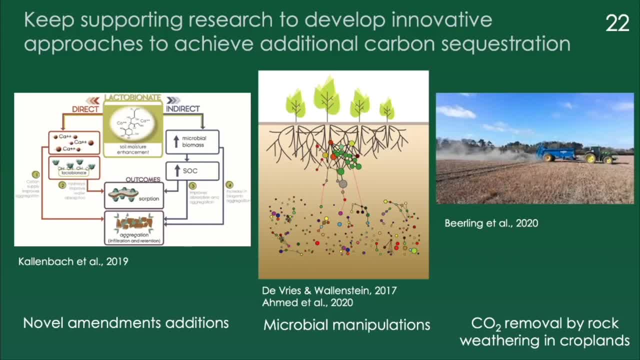 of the farmers. Finally, we need to still move the research forward because, as I stressed multiple times that we do have to know how to start today, We also have to keep doing research so that we can find innovative solutions that can potentially sequester even more carbon or increase the permanence of the carbon we sequester. 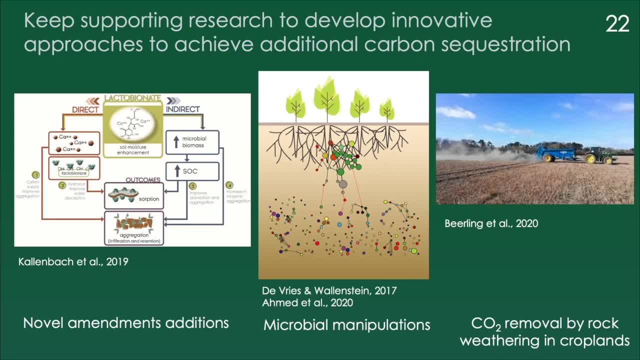 And so, for example, CSU, Matt Ballenstein and others are working in collaboration, which is industry of all kinds, to, for example, study how lactobionate might have a role in carbon sequestration, And you can imagine many other side products that could have similar effects. 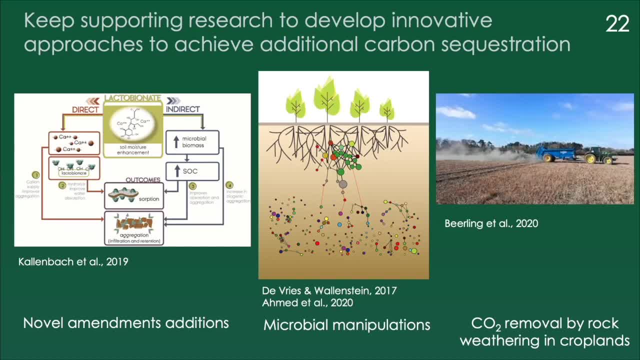 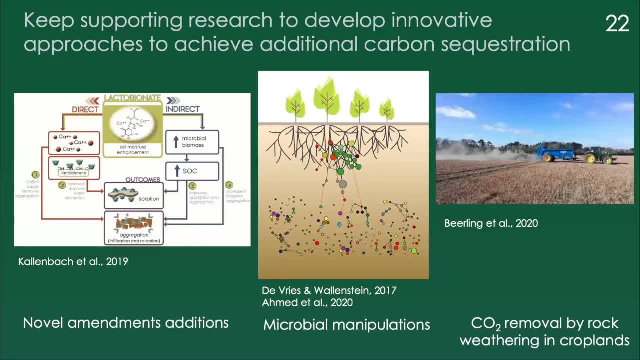 understand the role of carbon sequestration. We need to understand the role of carbon sequestration And the role of carbon sequestration is important in improving the connection between plant and soil microbiome to increase that efficiency And that can also be important. 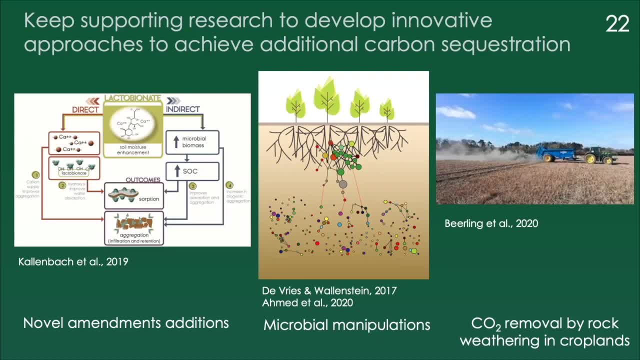 in increasing the tightness between the nitrogen and the carbon cycle and make carbon sequestration more effective, also in terms of not using the nitrogen. And some of you might have seen- I don't know an hour ago I told my last track of time. I think it was a month ago. 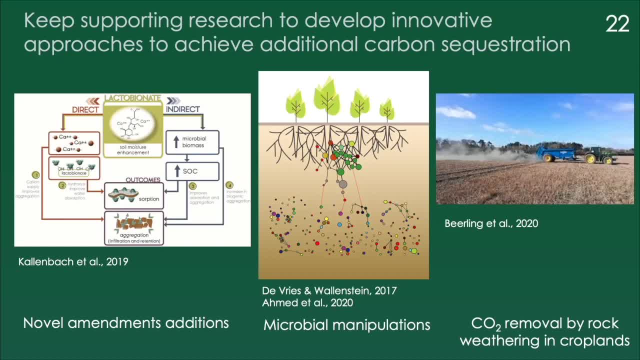 that came out in Nature people from a British group. they showed how we can actually sequester carbon by adding, possibly, silica rocks to agricultural soils, And so this is just to give an idea. but for sure, we still need to support research in a way that we can find innovative. 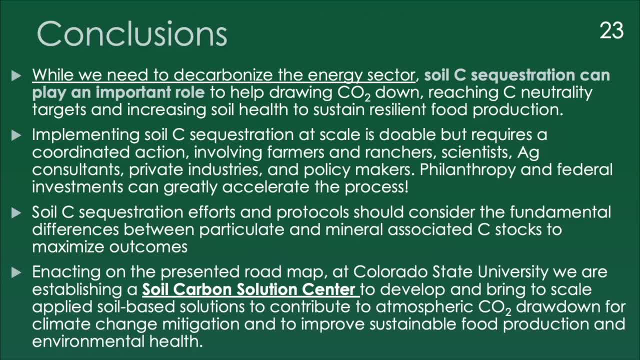 solutions. So in conclusion, I want to stress that again once more- I really love the fact that we keep stressing this- is that by no means what we are saying has to take away from the need to decarbonize the energy sector So that soil carbon. 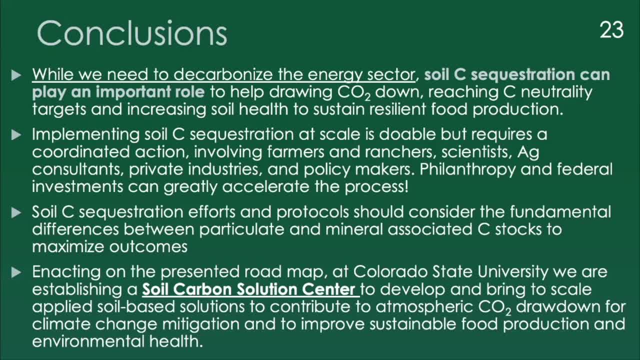 sequestration can play an important role to help throwing CO2 down, in particular because we have that very short time scale and also because carbon sequestration has a ton of core benefits and can increase soil health and improve the sustainability and resilience of agricultural soil. 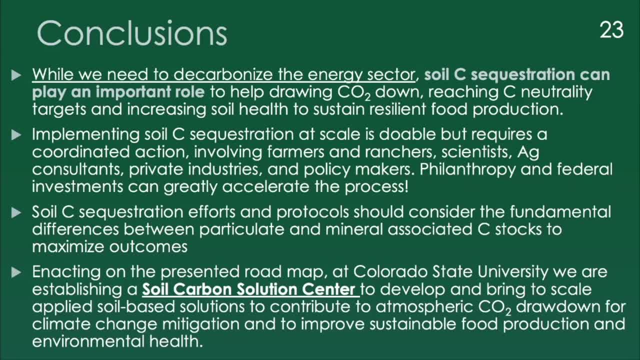 I think that implemented soil carbon sequestration at scale is actually doable, despite all the skepticism in this field, And I hope I have illustrated you what we should be doing or we can do in order to meet the most of those potentials. But we do need to work together and we do need to have again. 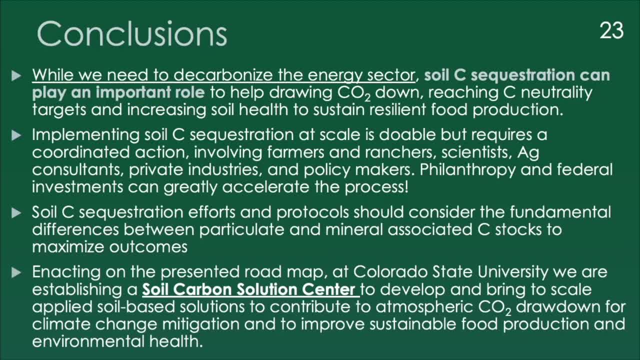 collaboratives between industries, practitioners, scientists and so forth. I do like to stress- and I know that I'm fighting back on that because people say: cost too much, the two puts is low, but it is important that we move, not just to. 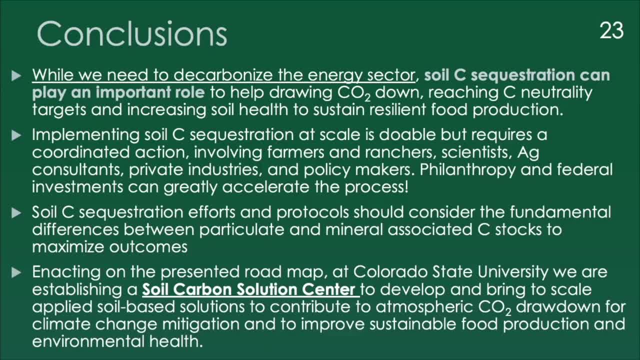 consider carbon one thing- and we might put dollars on carbon- that it stays in the soil only for a few years. It is important that we separate the carbon that might stay for longer and have a different function from the carbon that stays for a limited amount of time. 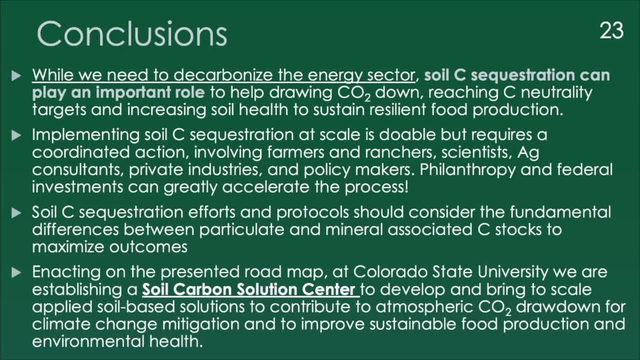 I'm very excited that the Colorado State University- we are actually enacting on this roadmap and creating a Soil Carbon Solution Center to to exactly create those collaboratives and start working on making those solutions a reality. With that, I'd like to thank all my group. 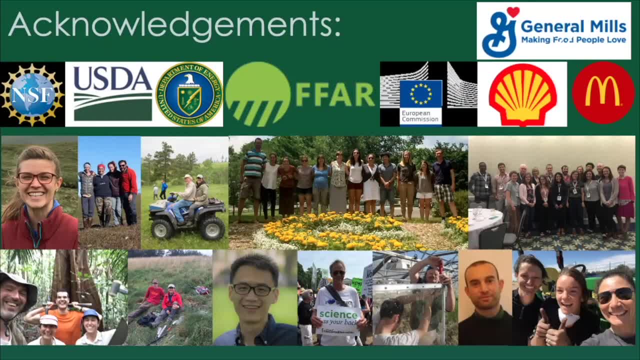 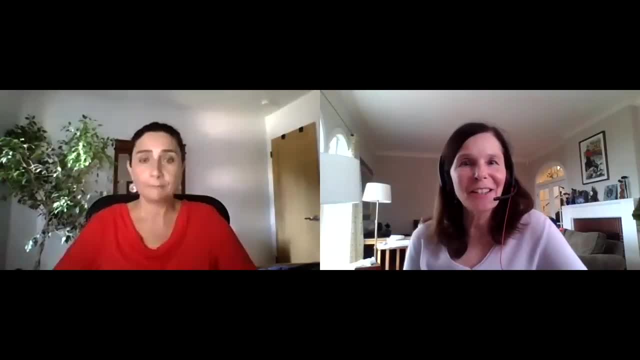 and great collaborators and all my funders and, of course, all of you for your attention, thanks. Thank you, Francesca. Great to see all that you're working on at Colorado State. I'd like to turn it over to Jenny, who is running the Q&A. 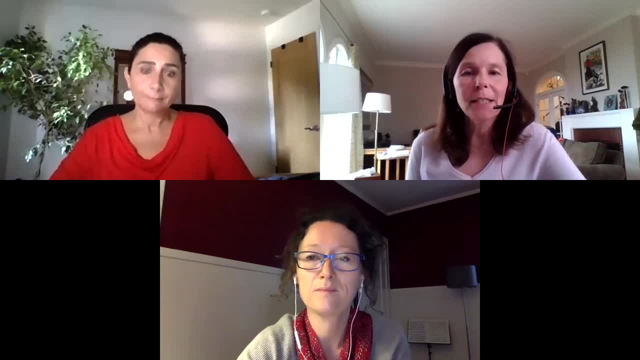 This morning. I can see we already have a number of questions that have come in. Please use the Q&A function at the bottom of your screen and continue putting them in, And Jenny will call on some folks to ask their questions now. Thanks, Sarah. 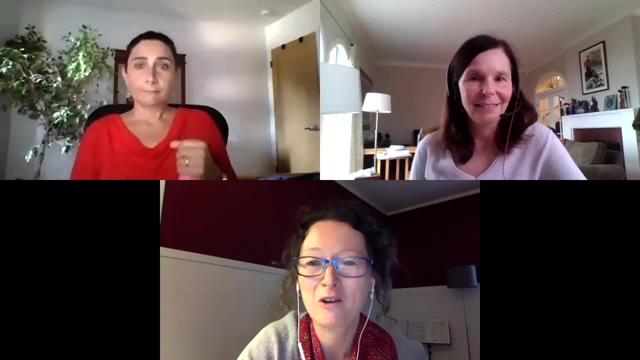 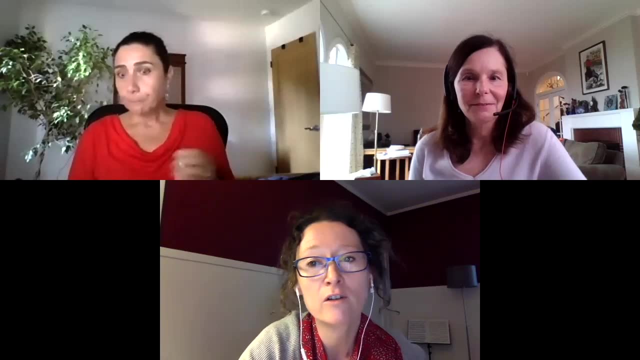 Thank you, Francesca. It was a lovely, wonderful, informative talk. We have a couple of great questions here. Laurie Weyburn, would you like to unmute yourself when you're able to and ask your question? One of the things I would be curious about. 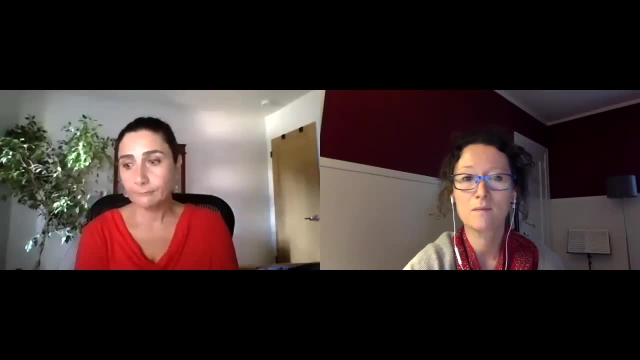 is. it does sound like organic farming and holistic range management approaches are really superior methods for enhancing soil carbon. Both they have lower inputs in terms of petroleum-based fertilizers, pesticides, et cetera, And they have enhanced soil organism populations, as contrasted with somewhat more intensive agriculture. 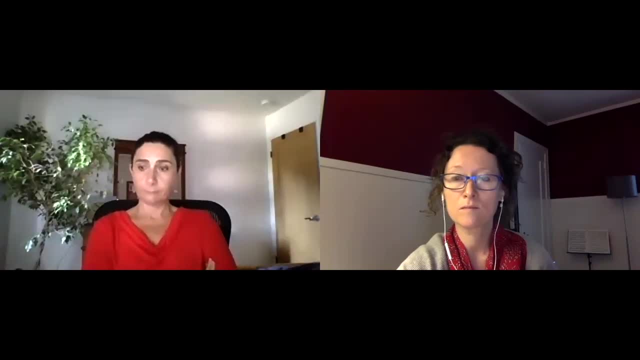 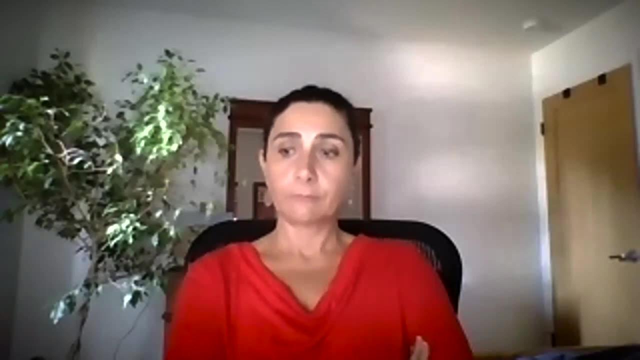 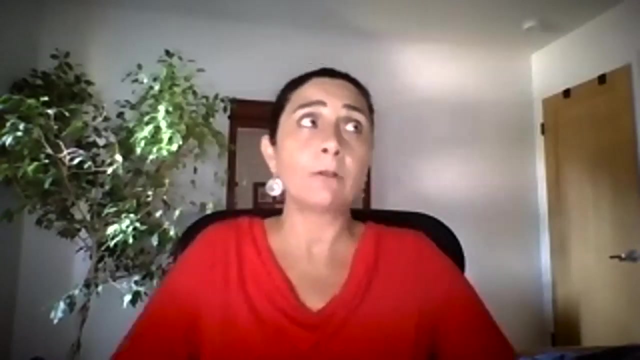 What does your research show about this And do you have any thoughts about impediments to broader implementation of that kind of approach? Yeah, I think you are perfectly right And actually we have been thinking about the fact that you need to diversify the rotation. 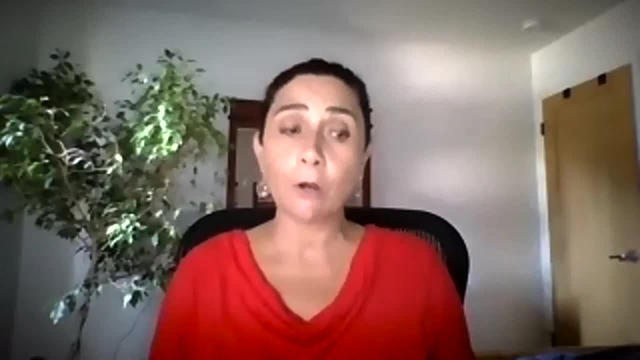 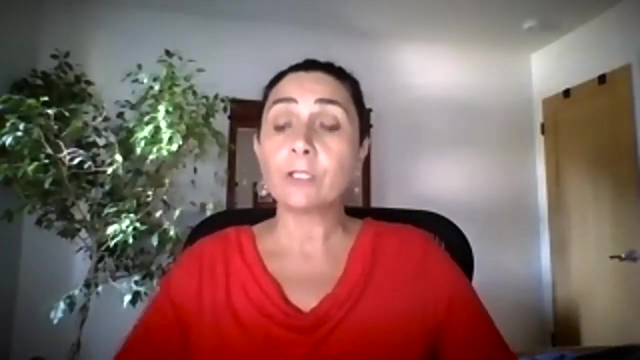 and increase the nitrogen input from legumes. But when we work at grain rotation, so without all the holistic regenerative approach that you mentioned, and just maintain the continuous cropping and introduce legumes in the crop rotation, we actually didn't have the same results. 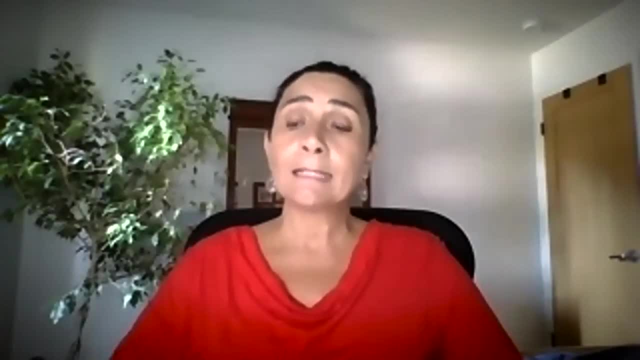 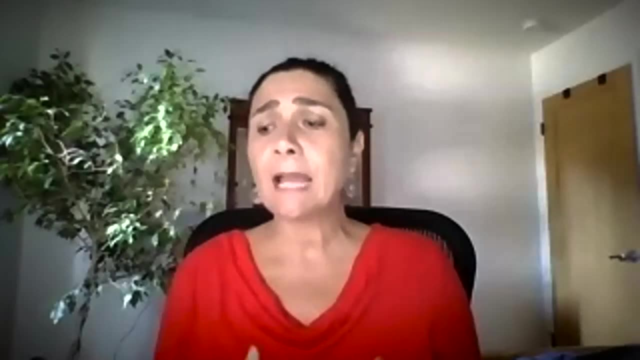 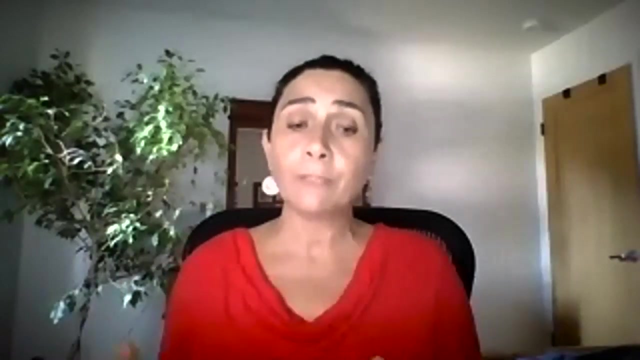 as the holistic approach, And that's, I think, is because, for example, the legume have low productivity as used as a grain, Like if you have a pea crop. that's, I think, very normal. um doesn't actually have the same amount of input. um, and and also the stage of the. 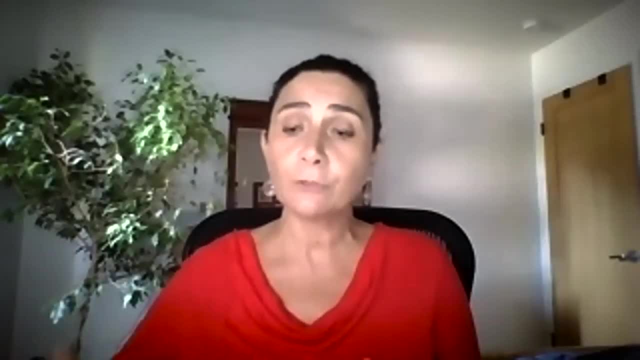 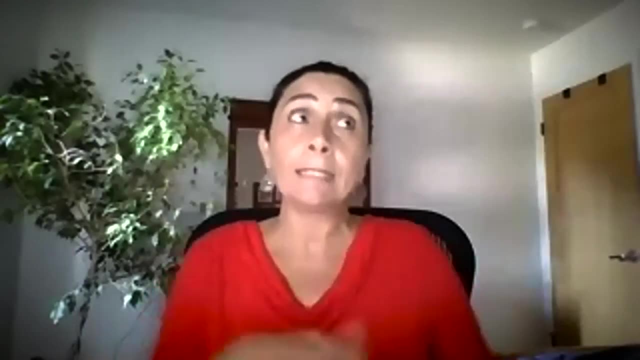 introducing um perennial stages and diversify the root inputs, um, those are all great things, that only the holistic management and the introduction of animals in the rotation um really move the system to a different level. so, um, i i do start to believe, uh, that to have the very announced response responses and not just move the needle to a little bit. 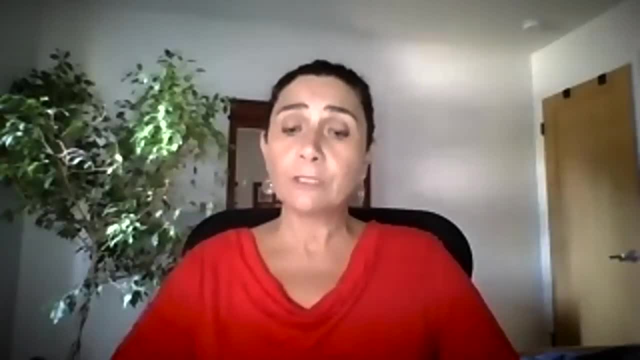 um, the most successful, also for the economics of the farmer um, is to go into the holistic. how much that much the economy of agriculture today, it's hard to say and maybe that's something that dave can speak to better, but but from a soil standpoint the holistic management is the best. thank you, uh. we'll take another question, uh, from the audience. 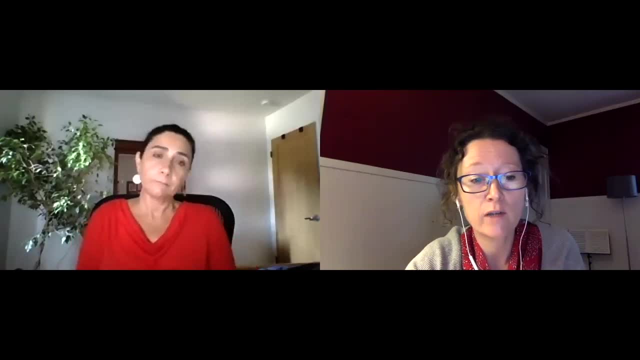 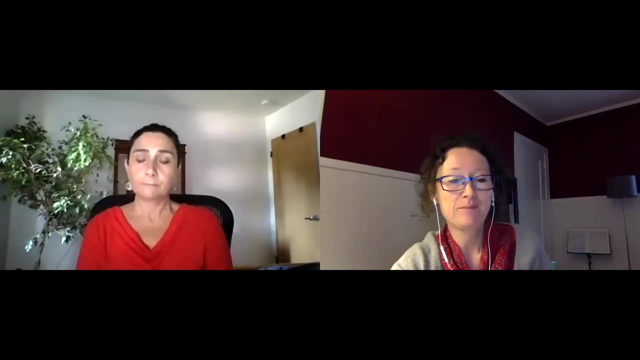 jessica, would you like to unmute yourself when you're able to and ask your question? sure, can you hear me. yeah, thanks, great, yeah, that was a really really great presentation. thank you so much. um, you know, i found the map of the european forestry space in palm and ma'am really fascinating and, in particular, you know the. 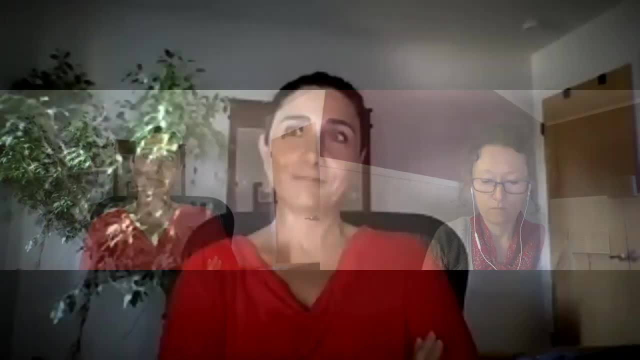 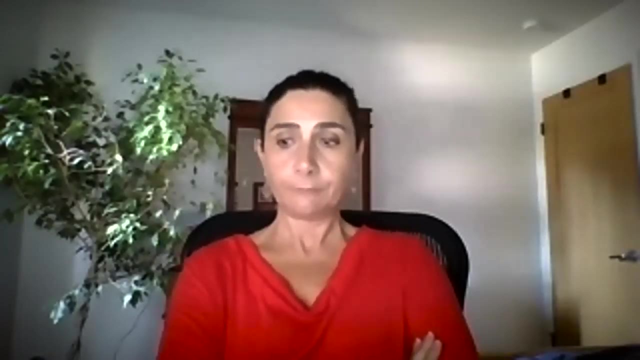 fact that there's this abundance of palm in coniferous forests, for example, and in thinking about implementing nature-based solutions and considering that many of the common pathways are in the forestry space, i was wondering what your opinion is of possible amendments to forest soils to either increase the ma'am concentration or somehow increase the recalcitrance of palm in. 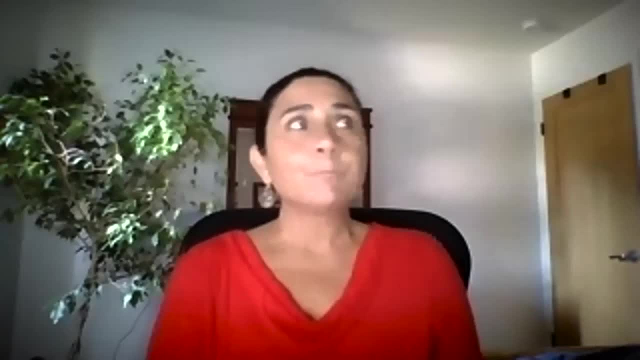 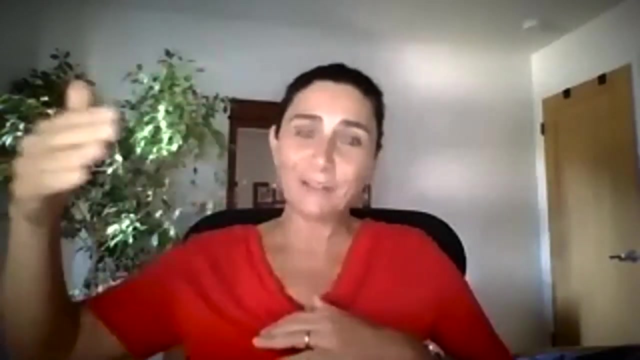 forest litter and soils. um so it it also depended on the, on the soils, of course, and and one thing i want to press uh to to make sure, is that we are talking about the mineral soils, not the organic layer, because on top of that, there is a huge amount of organic material that is even more vulnerable. um the the point to consider. 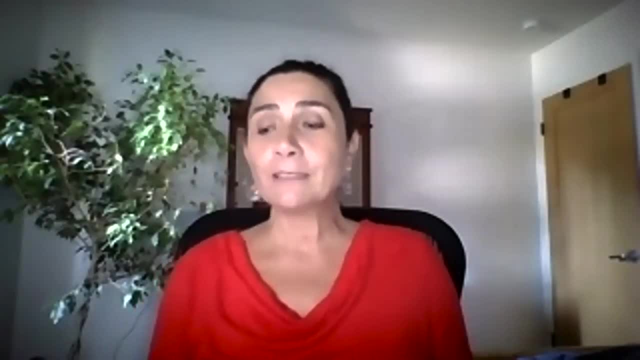 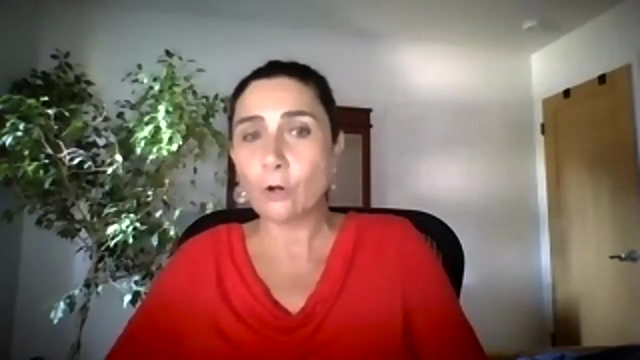 is that, at least in europe, for us, given the long history of land use, forests are the most sandy and acidic soils of europe. um, and, and, and. so there is this uh connection between uh, the land use and the soils, and and how much you know you can, you can do with that. 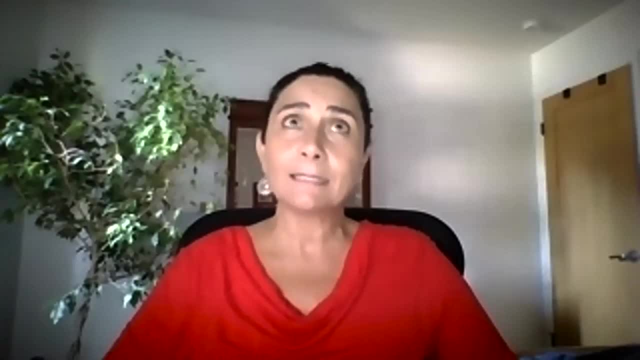 um. now i think that um, and the other thing is that conifers only associate to ectomycorrhizal- that also um, are prone to form more um palm rather than than ma'am. so there is an inherent limitation on how much ma'am you can. you can sequester in in um in forest, um. 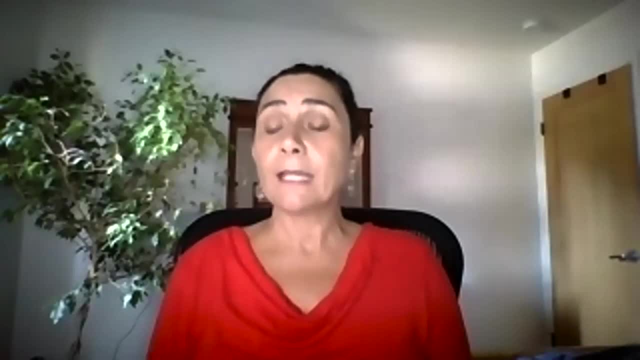 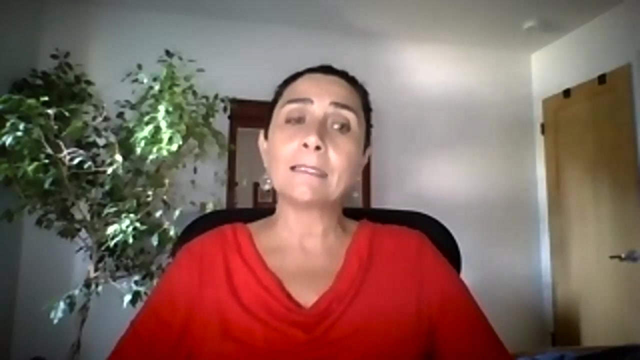 you can work um with, again trying to diversify the forest because, for example, the deciduous forest are actually much more similar to the grasslands than they are to the conifers and and and some deciduous, mixed deciduous forests can also have um more abuscola mycorrhizal. uh, that can promote my own formation, and so i i think that you know. 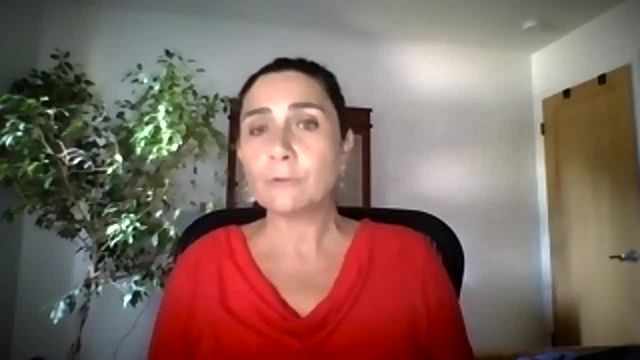 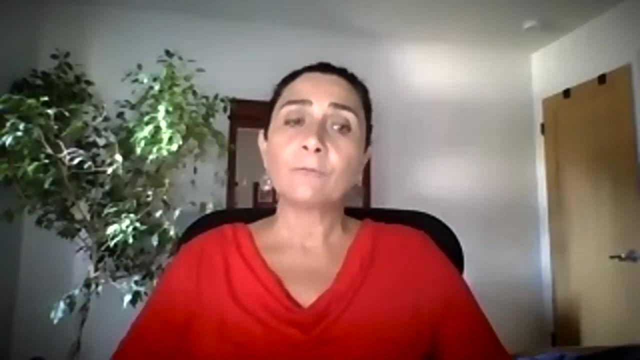 for established coniferous forest. there is so much you can do um if you are regenerating forest um and and afforesting, it's important to understand what's your soil, what's the potential, and design a forest that possibly is a mixture um so that you can accrue. also, ma'am to having more deciduous and. 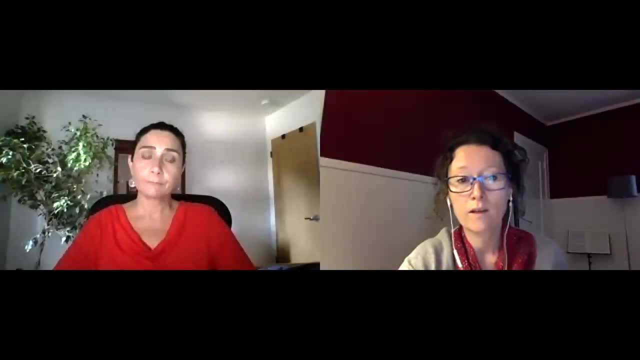 to have more abuscola mycorrhizal too. thank you, i'm hoping we have time for one more question. we have a lot of questions that are we probably won't get to, unfortunately. so, um, christian davis, would you like to go ahead and 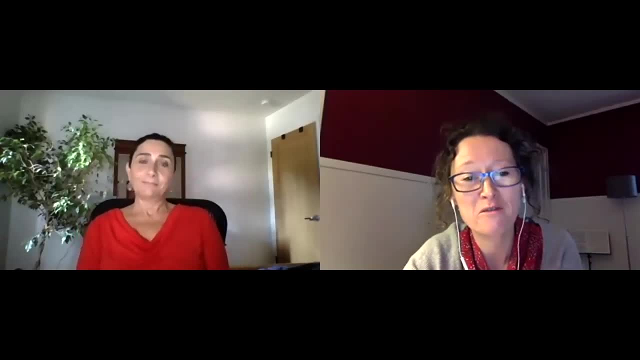 ask your question once you're able to, uh, unmute yourself. yeah, hey, francesca, thank you for a really brilliant presentation. i think a lot of the work you have done and are still doing in terms of mechanistic understanding of how soil carbon accumulates is really kind of pushing the boundaries. 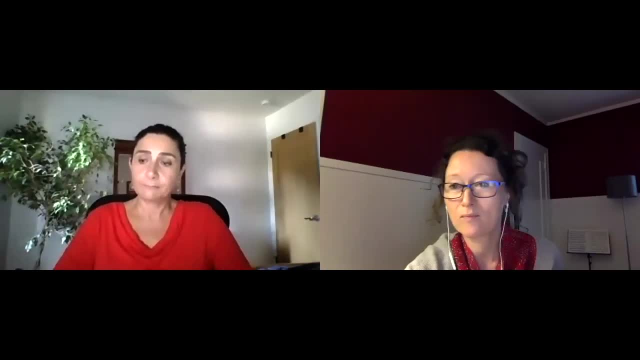 of the field. so thank you for doing that. um, do you have some idea on how far away we're actually going to be able to, how far away we are from being able to manipulate, uh, the processes to drive and increase carbon stocks? and do you think we're, in the future, we may be able to get to a point where 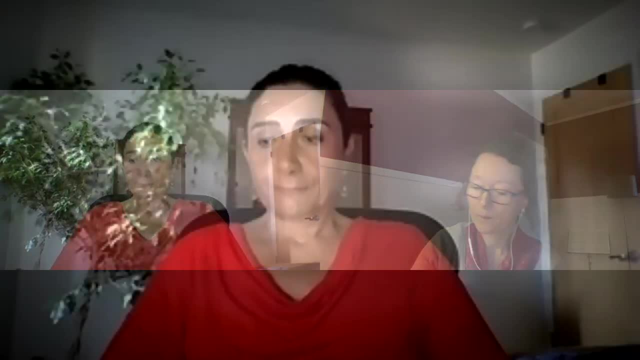 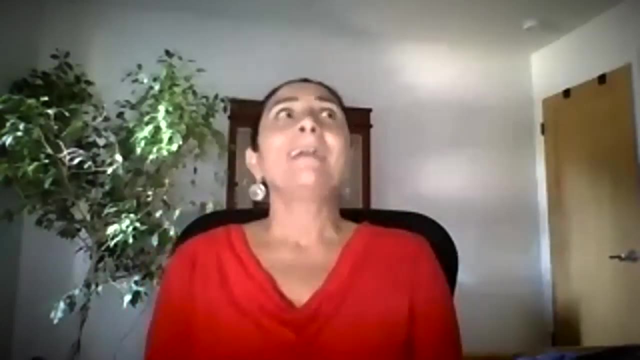 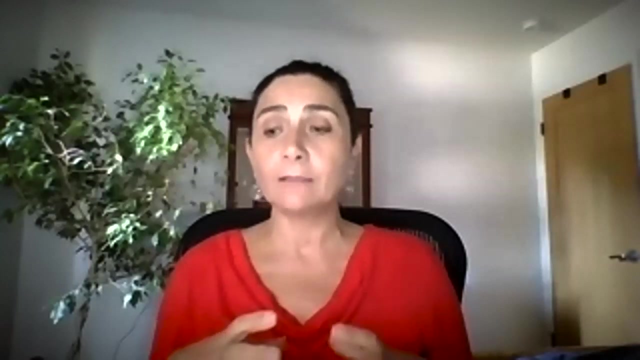 we can just analyze a sample and kind of propose a tailored solution, uh, to farmers in the future. yeah, so i i'm actually not a strong believer of the um, so i do think that microbes are the, the engine that really drive how much stays and how much goes and uh, what, what, how much form. 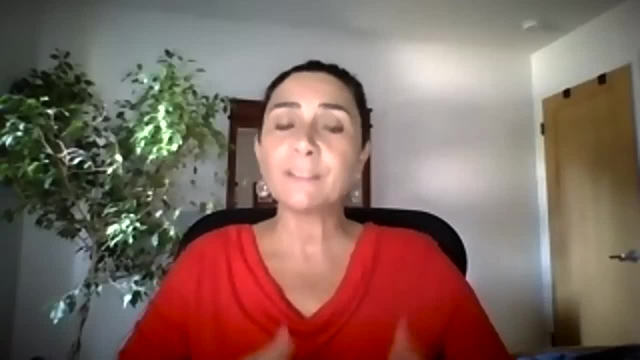 is formed, how much mayom is formed? uh, but they respond to the, the, the management, and to the plan, and and so, in my opinion, again actually going back to the holistic um uh method, i think that we are not far from creating a very integrated plant microbe relationship, and you can get that by um 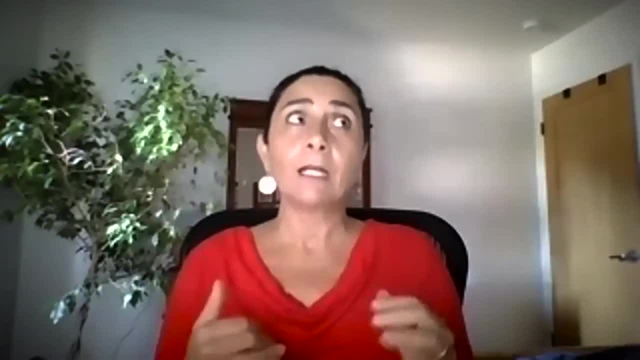 by, by basically um having, um, the, the mutualism that we see, natural system, where the fungi bring the microbes bring the nitrogen, uh, either by fixation or by scavenging to the plant and the carbon, and the plant provide the carbon. so if we stop fertilizing with 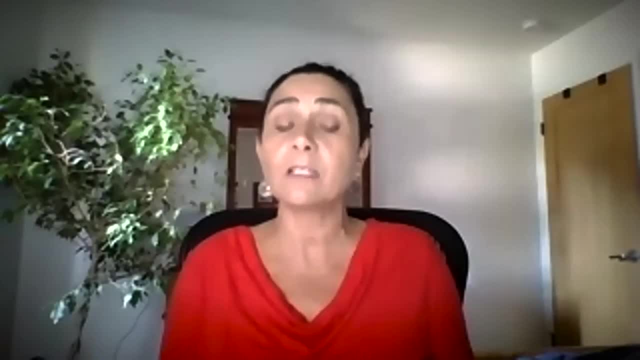 we start promoting that plant microbial interactions, we are a long way there. the other thing we need to do is to have more roots and deeper roots. plant breeding has been done so that our crops have an absurd shoot to root ratio, with roots that are unexistent, and so we need